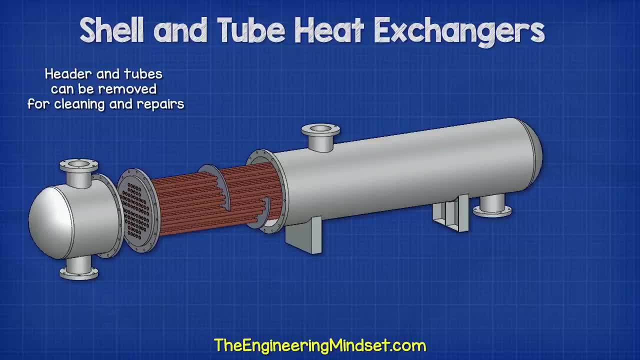 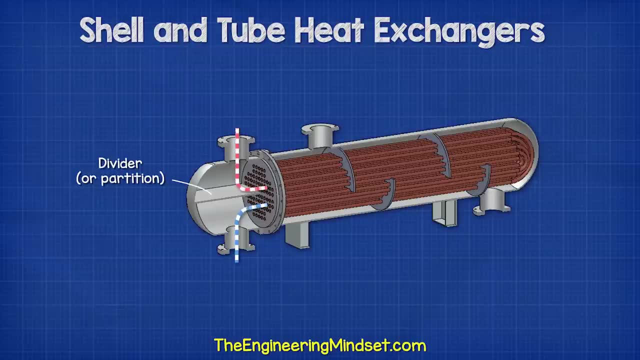 The header, as well as the tubes, can be removed for cleaning, repairs and maintenance. Inside the header is a sheet of metal known as the divider or the partition. This separates the tube ends, enabling the fluid to flow into and then out of the heat exchanger tubes. 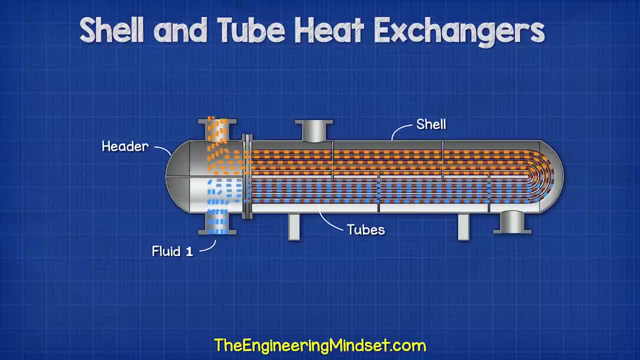 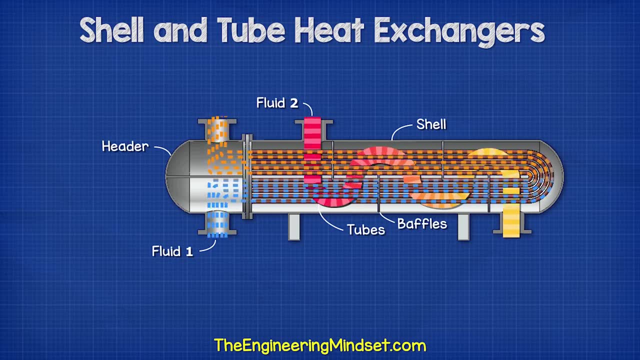 Fluid 1 will flow through the header into and around the tubes, then back to the header. Fluid 2 will enter the shell and surround the outside of the tubes. The baffles will partially block the flow, which will force the fluid to turn multiple times. 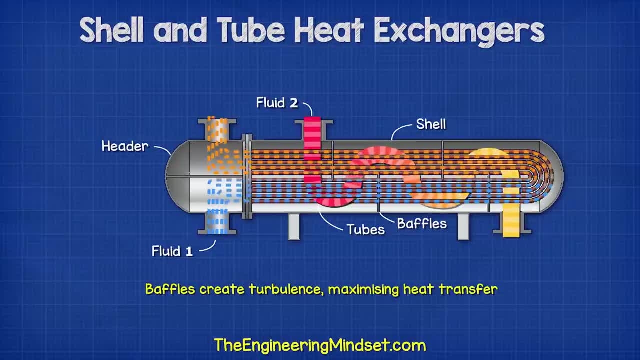 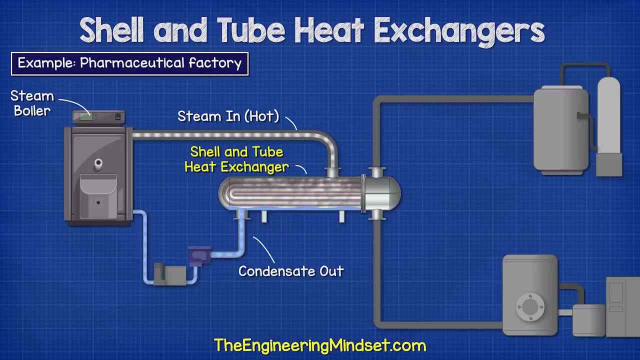 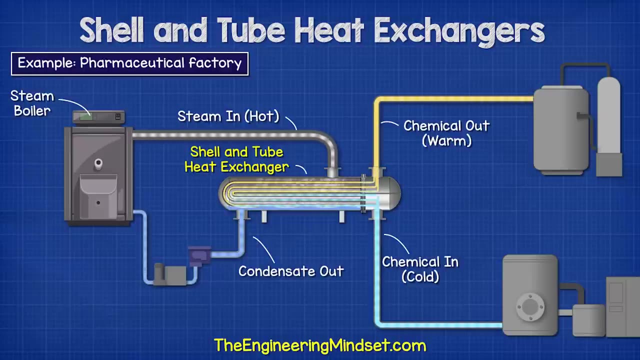 This creates a turbulent flow and ensures that fluid 2 mixes with itself, which ensures maximum heat transfer. For example, we might find this in a pharmaceutical factory with a boiler providing steam into the shell which surrounds the tubes. A chemical product is then pumped through the tubes and this absorbs the heat of the steam through the tube wall. 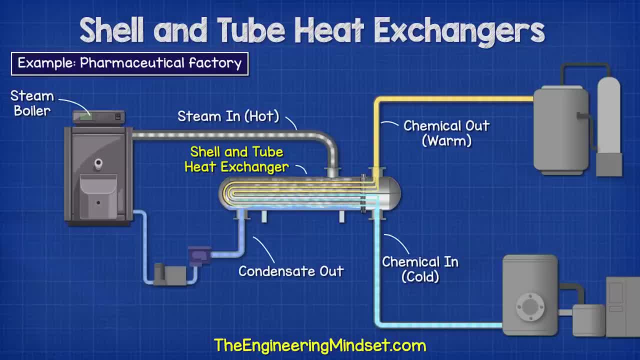 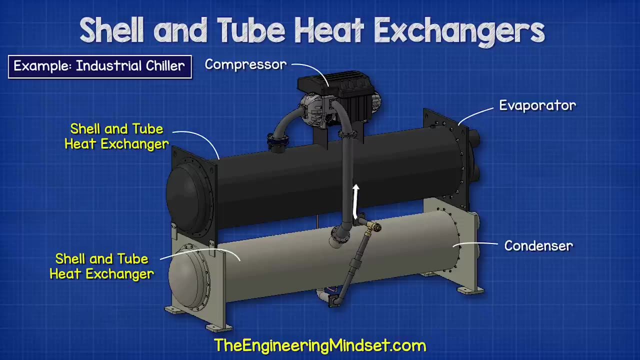 So this product is going to exit the heat exchanger much warmer. Meanwhile, the steam will start to condense into a liquid and flow back to the boiler to pick up more heat and repeat the cycle. Additionally, these are used in refrigeration applications like this industrial chiller. 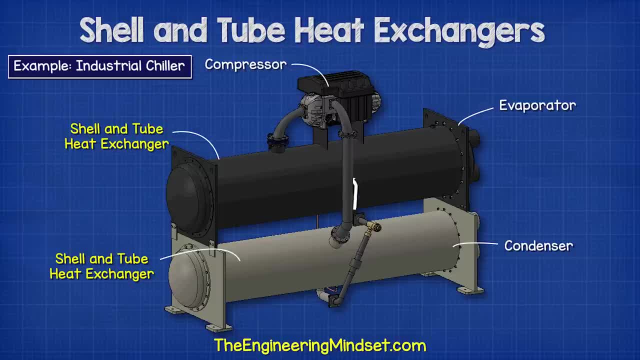 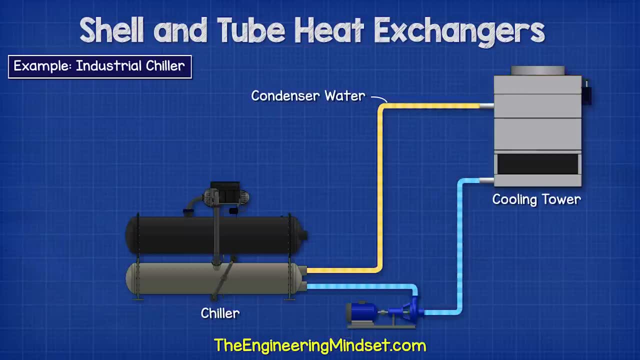 We have the water flowing through the tubes, then the hot refrigerant in the shell. The water will absorb the heat of the refrigerant so that it can transport this to the cooling tower where it will be ejected into the atmosphere. The water returns cooler to pick up more unwanted thermal energy from the chiller. 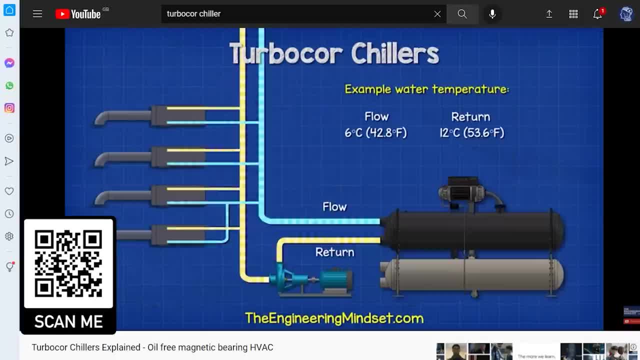 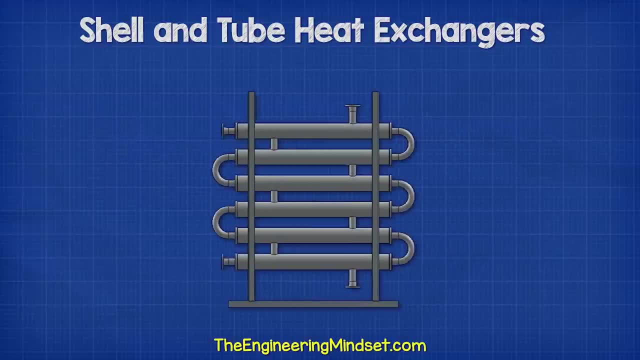 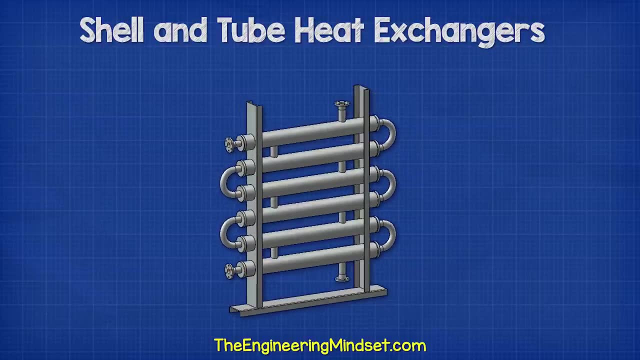 We have covered how chillers work in great detail previously. Do check those out. I'll leave a link for you in the video description down below. Double pipe or tube-in-tube type heat exchangers will look something like this. This is similar to the shell and tube heat exchanger. 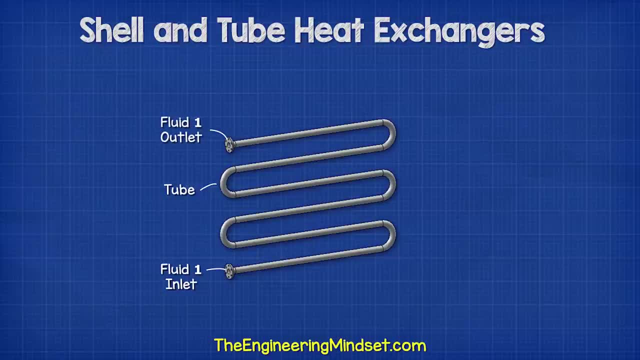 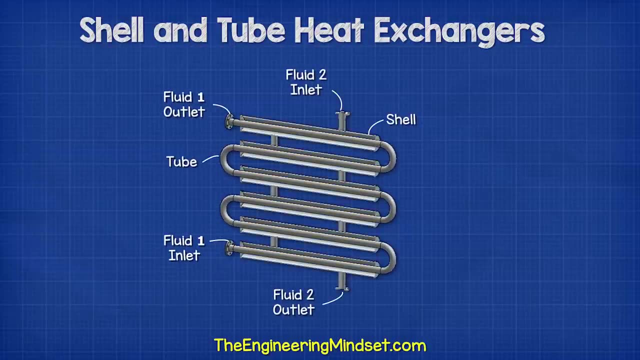 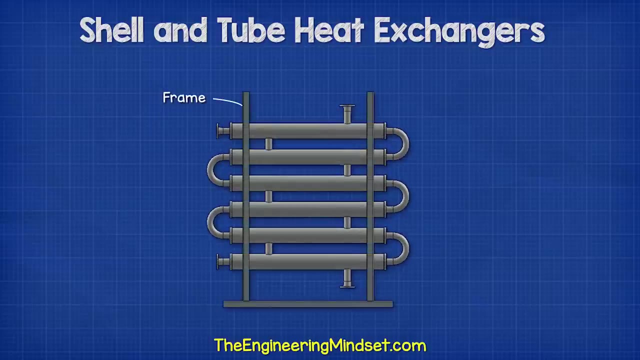 because essentially we just have a tube which runs back and forth a number of times between an inlet and an outlet. This is surrounded by a shell which has another inlet and outlet. A metal frame will hold the unit in place. Typically these will all be made from stainless steel.